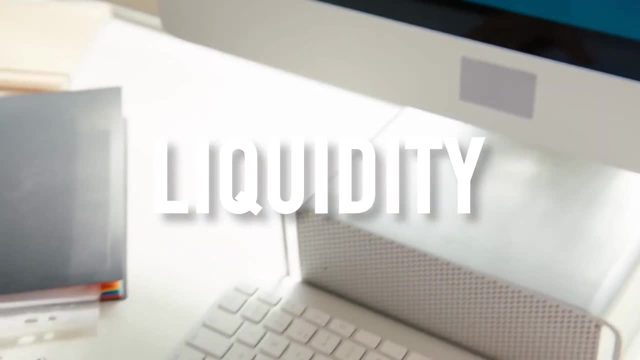 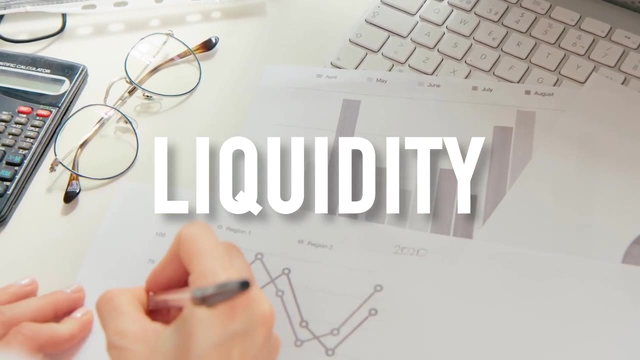 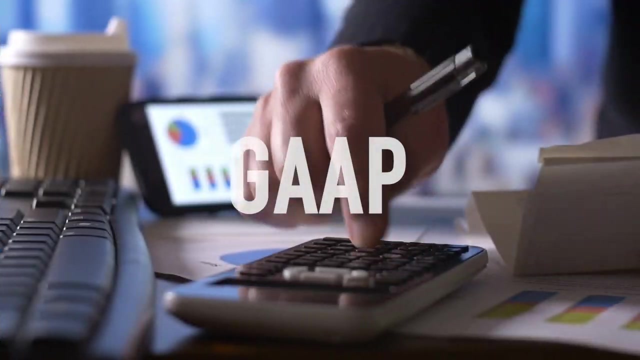 equity. Liquidity is the principle of how quickly an asset can be converted into cash. Cash is the most liquid asset, usually followed by stocks. The least liquid asset are land and real estate, because it can take weeks, to months, to years to sell Gap. no, not the store, but generally accepted. 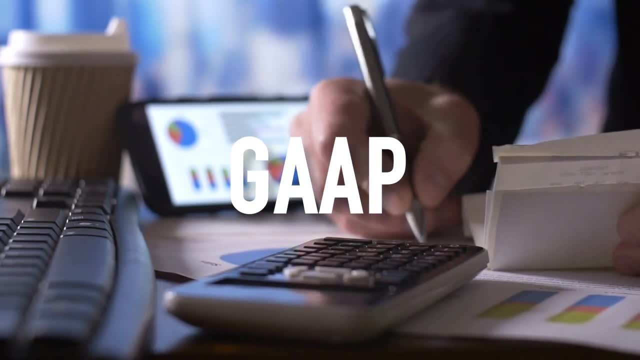 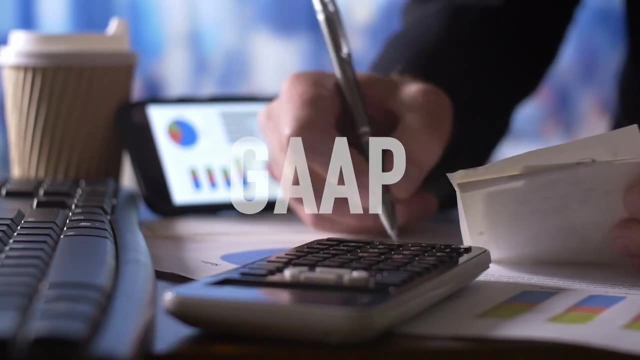 accounting principles are rules and conventions that govern how a company reports the state of their finances. It's essentially just a standard, and companies can report their earnings as gap or non-gap. Capital gains are just the increase in value of an asset above what you paid for it. 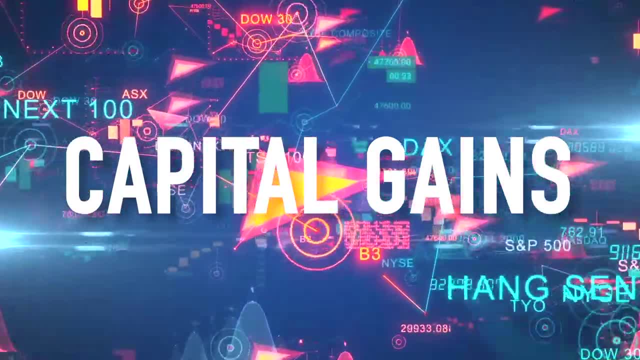 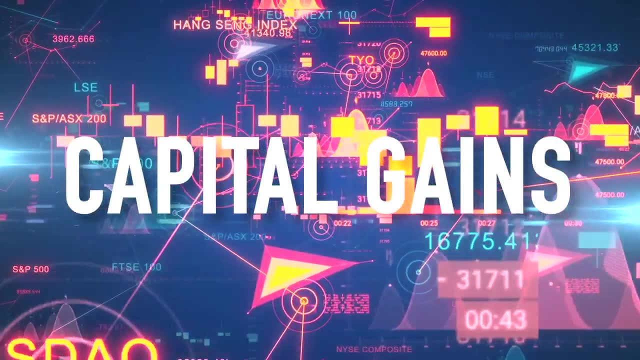 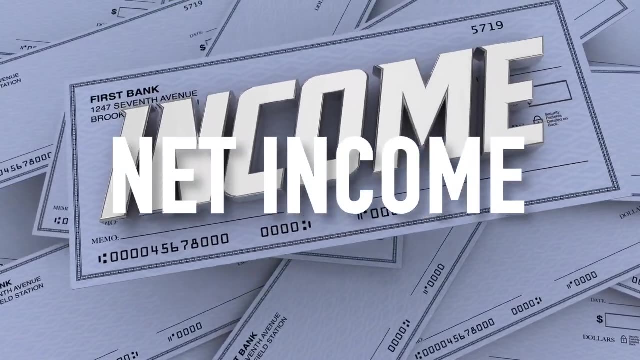 Capital gains can be realized and unrealized. Unrealized gains mean the asset hasn't been sold, and realized means it has You pay taxes on. realized capital gains and capital losses are the same, but when the asset is worth less than you paid, Net income is just total revenue minus expenses. Equity is just the. 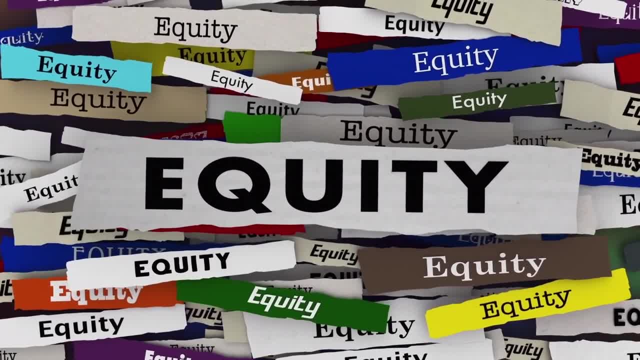 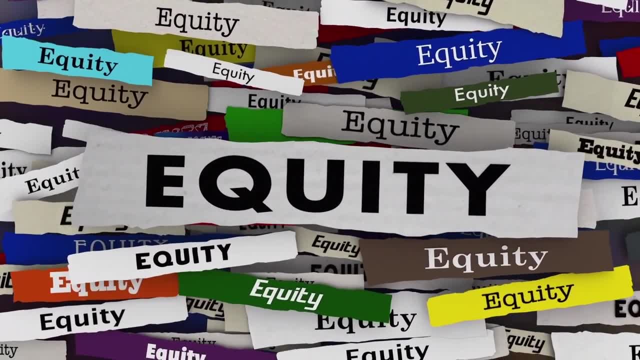 amount of money someone has in a stock or asset after subtracting off debts and money owed. It's possible to have negative equity, like in a car or house, if you owe more than the asset is worth. Often, a cause of negative equity is depreciation, which is a simple decrease in an asset's value. 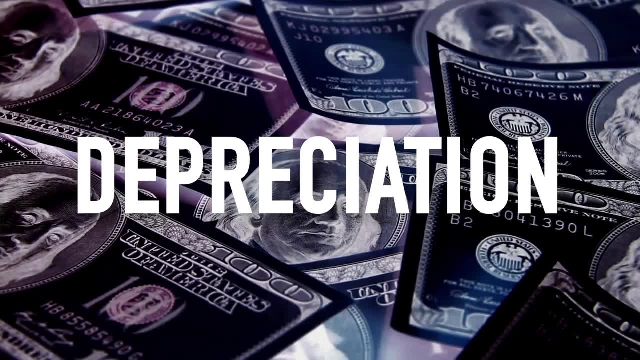 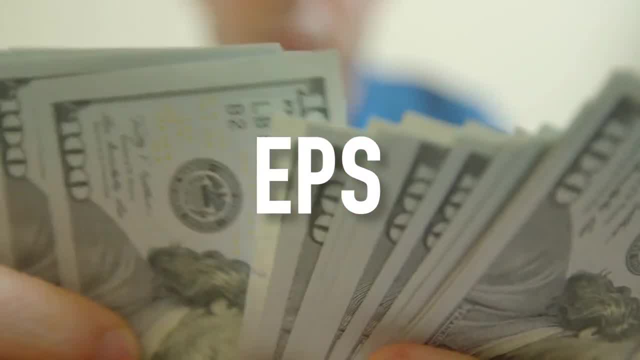 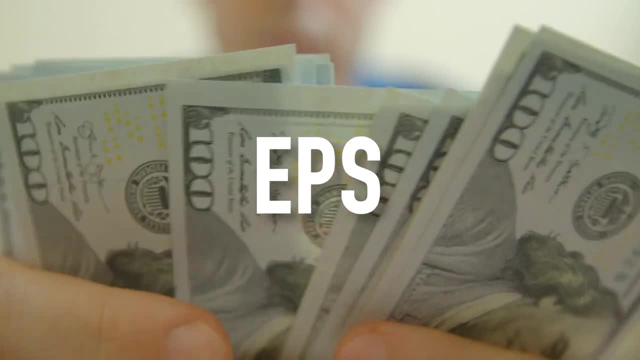 over time. Physical assets depreciate over time, with real estate being the usual caveat to this rule. EPS, or earnings per share, is the usual way in which a company's profitability is represented. It's simply net income minus dividends divided by the number of shares- Usually share prices for a 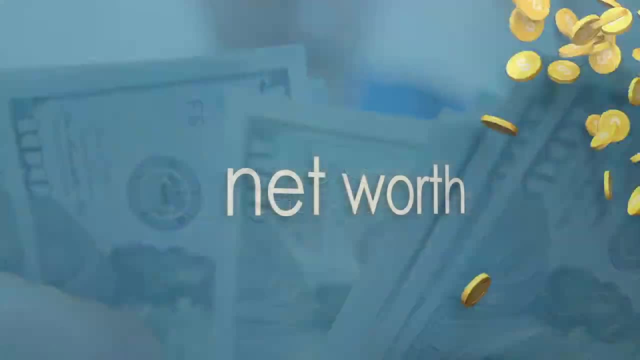 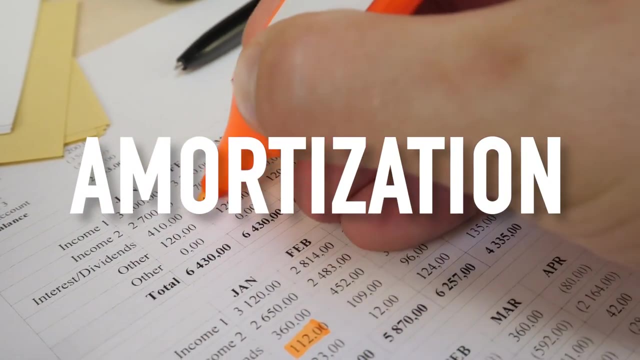 stock end up being some higher multiple of EPS. Net worth is just the value of everything you own minus what you owe. Amortization is just the process of accounting for an asset that is intangible or non-physical in a way that's more than what you own. It's basically a lot of what you'd want. 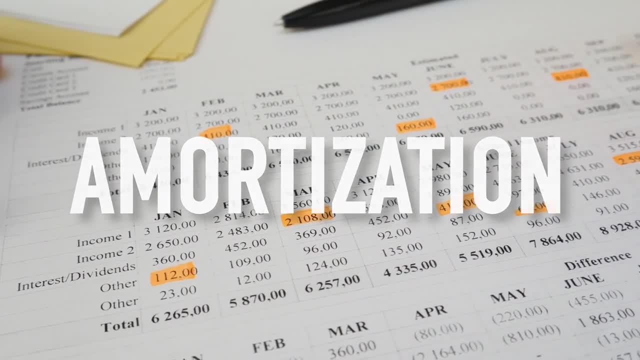 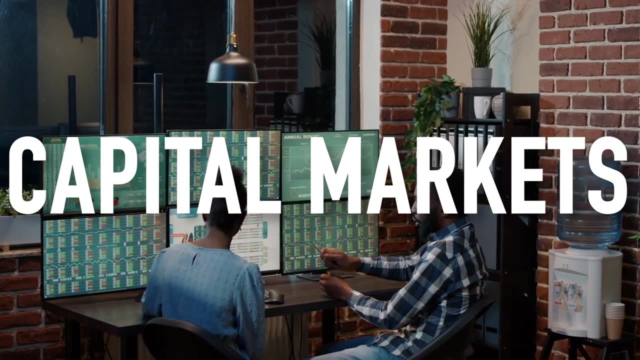 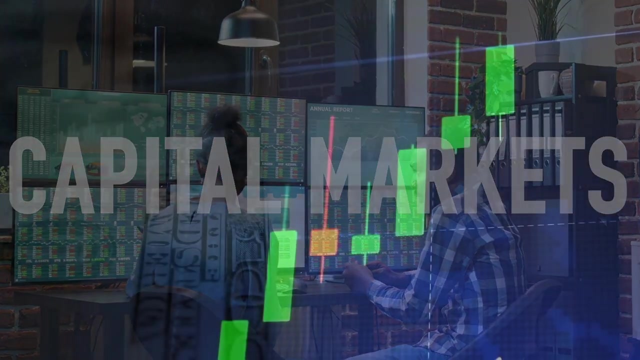 This usually applies to assets like patents, copyrights or trademarks. Capital markets are simply markets where buyers and sellers trade financial assets. Companies, institutions, mutual funds and hedge funds are the usual participants in these markets. Profit margin is just net income divided by revenue. This gives companies an indicator. 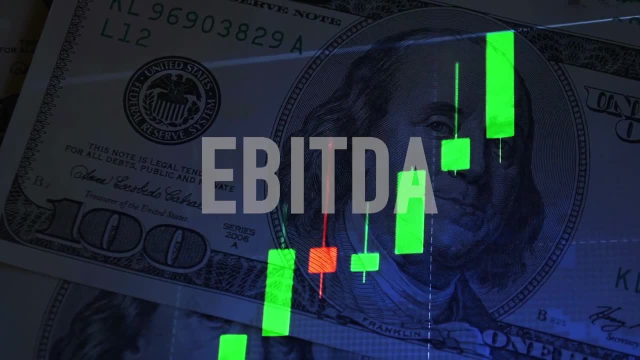 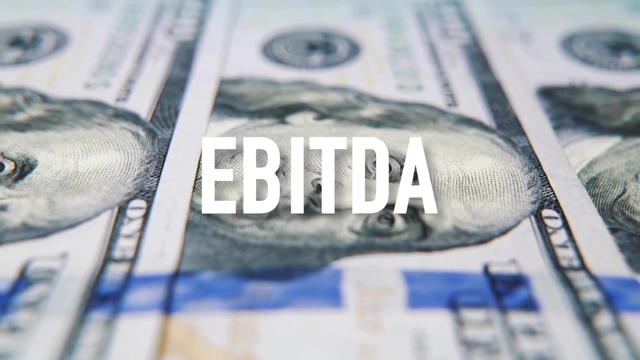 of how much wiggle room they have to continue turning a profit. EBITDA, or earnings before a mortgage, is a lot more competitive than for the stock to depend on Every house under a mortgage for interest taxes. depreciation and amortization is a term commonly used to describe a company's 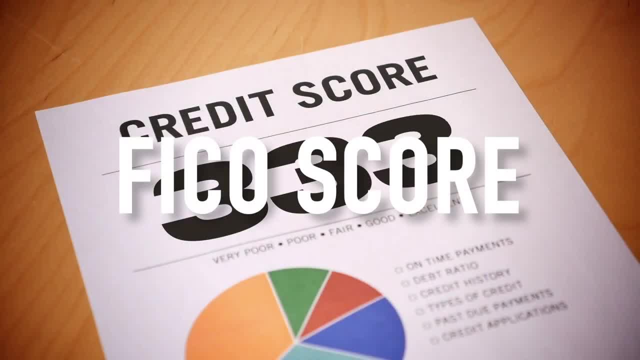 cash flow. FICO score is just a credit score from Fair Isaac Corp, the company that invented credit scoring. The score ranges from 300 to 850 and is based on payment history, length of credit and total amount owed, though no one knows the exact formula in the public. 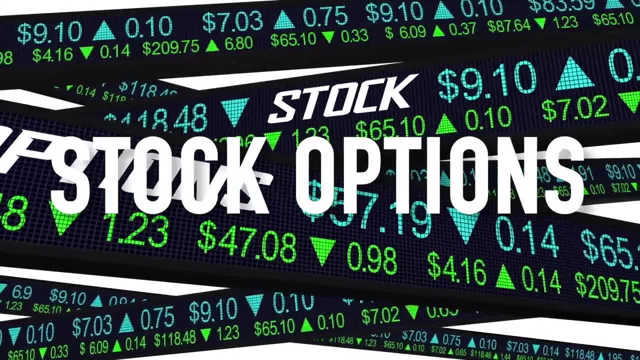 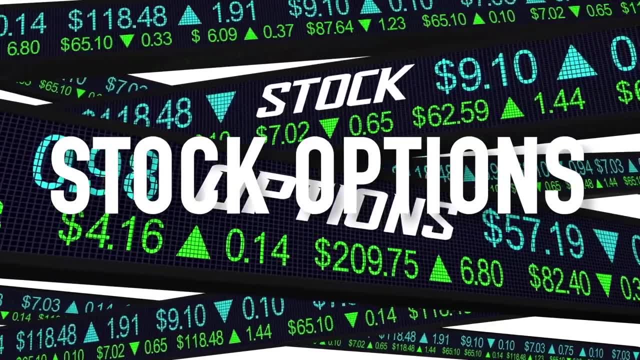 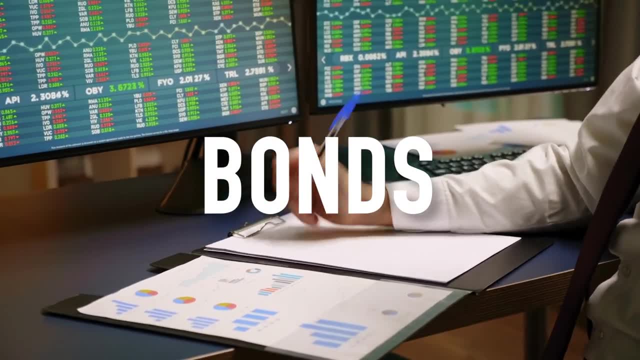 Stock options are the option or the right to buy a company's stock at a given price. These are generally given to employees and can be hugely valuable if a company's stock goes up after being granted an option at a lower price. Bonds are essentially just a loan from the purchaser of the bond to the seller of the bond. 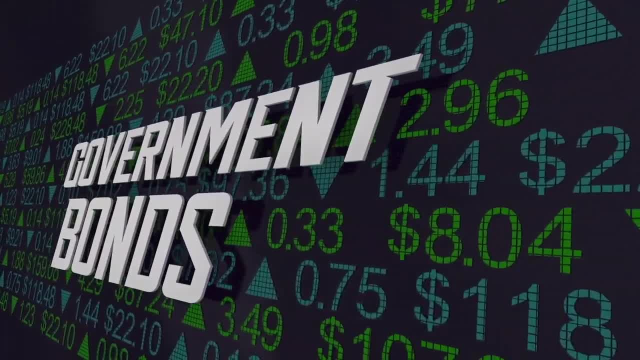 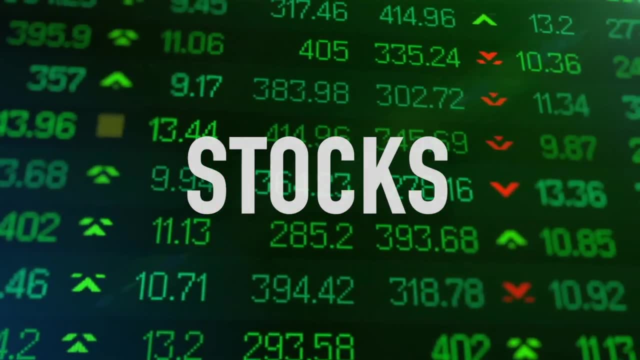 Government bonds are just notes for loans between the buyer and the government. Over time the government pays it back, but before then you can also sell the bond to other investors. Stocks are just shares or portions of a private or public company that can be traded or sold. 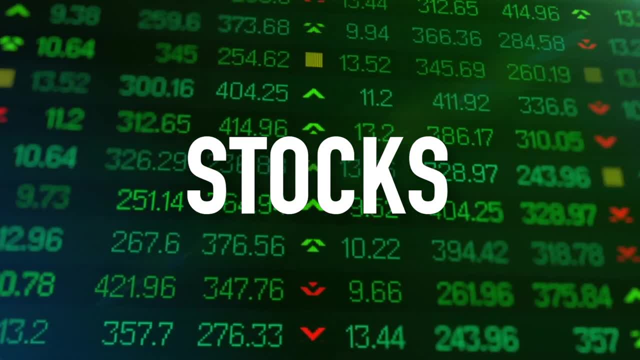 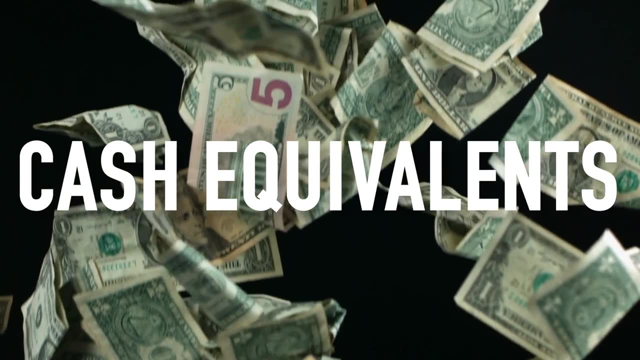 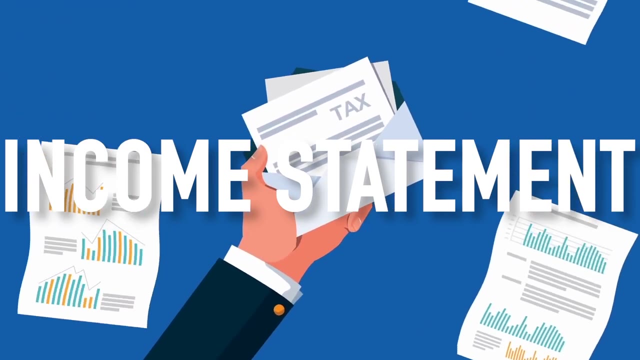 Stocks have value based on a company's earnings, potential earnings and other factors. Cash and cash equivalents refers to assets that are either cash or can be converted to cash easily, ergo they're liquid. An income statement is just a financial statement, summarizing how much income. 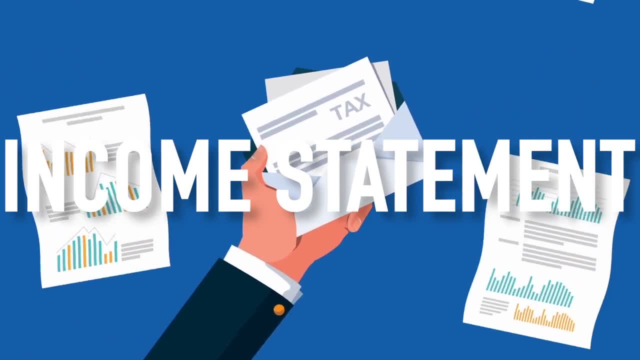 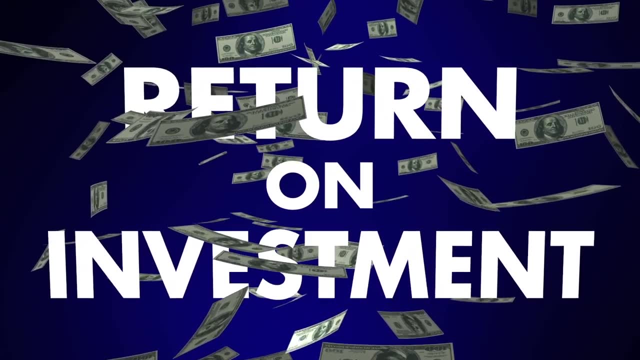 and expenses a company incurred in a given time, often called a profit and loss statement. ROI or return on investment, is a calculation that indicates how much money was made from an investment. It's calculated as a return on investment, but it's not necessarily a return on. 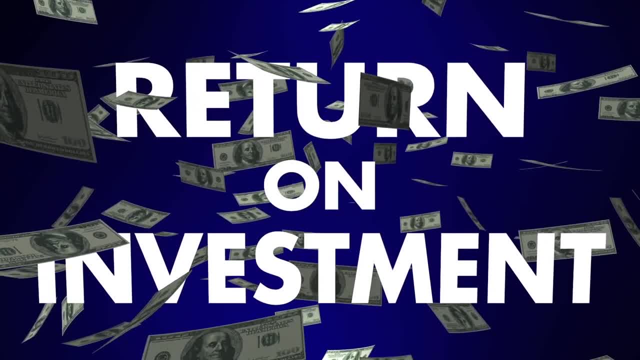 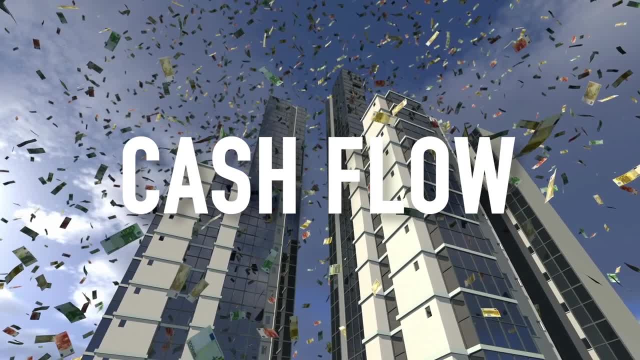 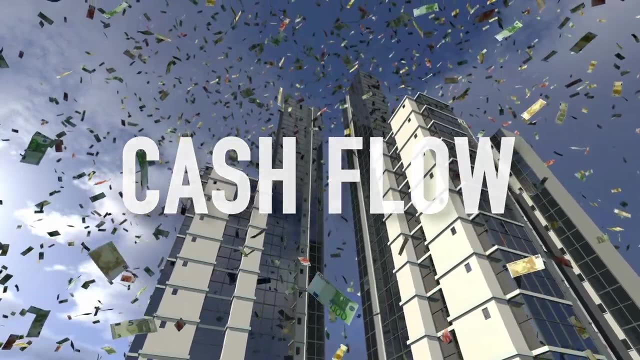 investment as the income minus the cost divided by the cost times 100.. In this sense, it's expressed as a ratio. Cash flow is simply the net balance of cash that is going in and out of a company. It can be segmented into operating, investing and financing cash flow, based on where the money 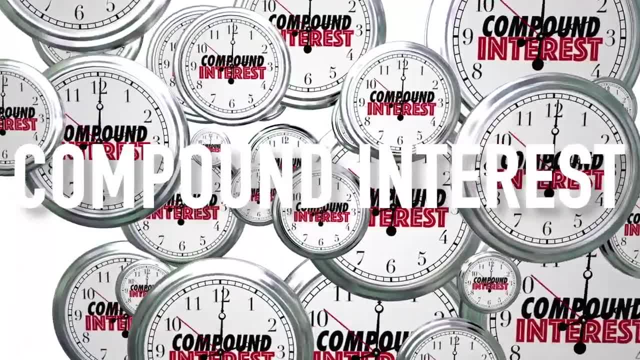 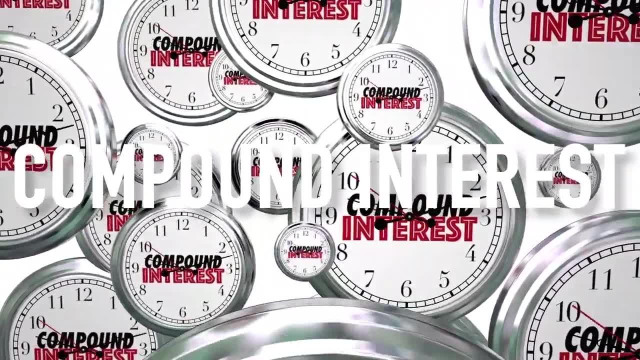 comes from. Compound interest is essentially just interest on interest Over time. after earning interest on an investment, that interest payment starts earning its own interest, compounding over time getting larger and larger. Valuation is just the worth of an asset or a company. Generally it's calculated with varying 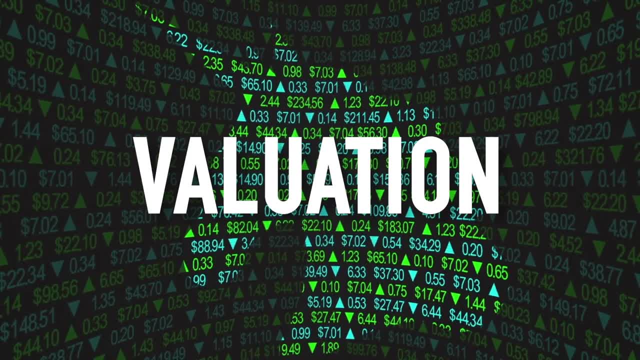 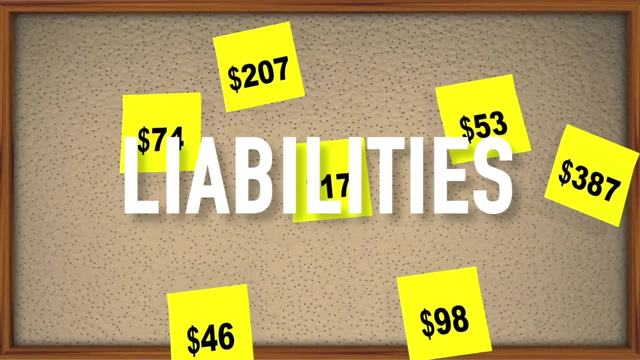 formulas incorporating income, EBITDA, revenue and cash flow and other financial figures. Liabilities are anti-assets or just debts. owed Liabilities can also present themselves as wages to employees or payments due to suppliers. Working capital is the difference between assets and